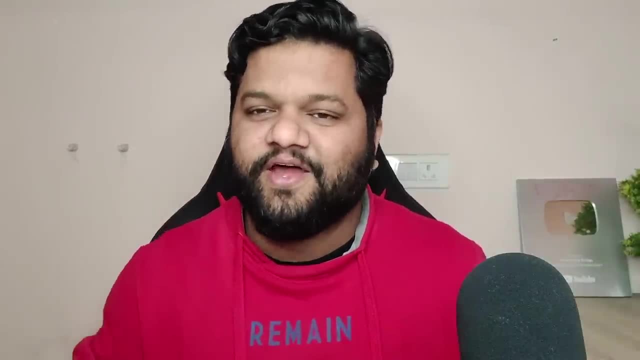 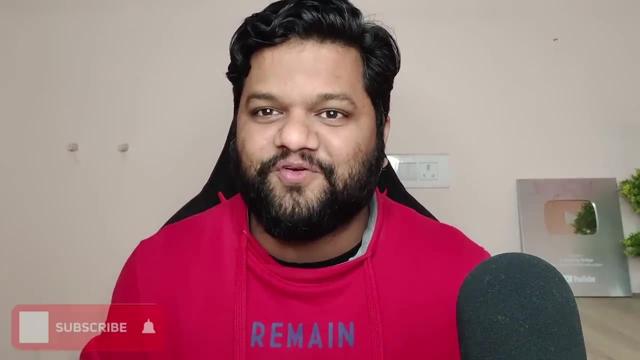 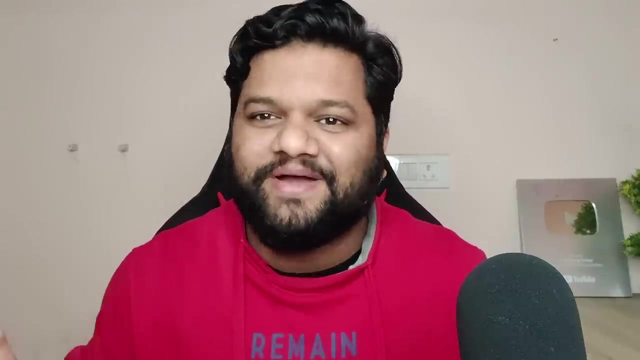 Hello data lovers, So I hope you all are doing super amazing. Well, it's 2023. And if you remember, two years back, I created one data engineering roadmap video on my channel and you guys just loved it And I even think that was something very, very informative I created. 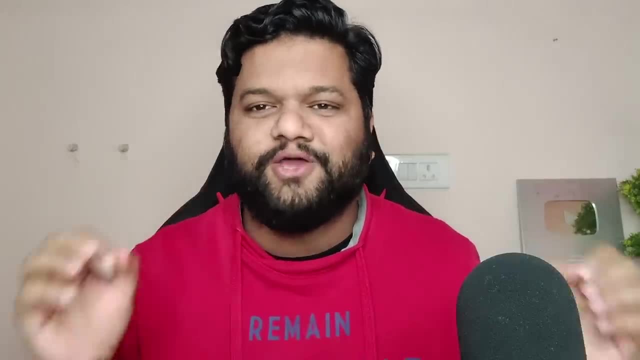 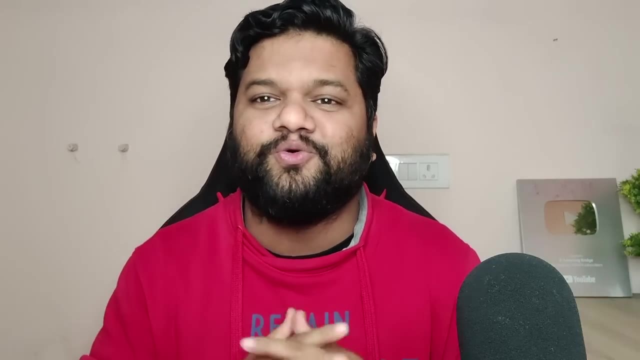 on my channel for the very first time. So in this two years of gap, I also learned a lot of new things in data engineering, explored a lot of new tech stacks as well, So I thought: why not to create a newly, freshly upgraded version of data engineering roadmap, or basically: 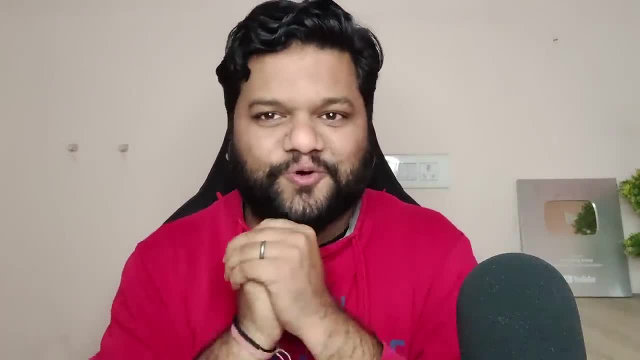 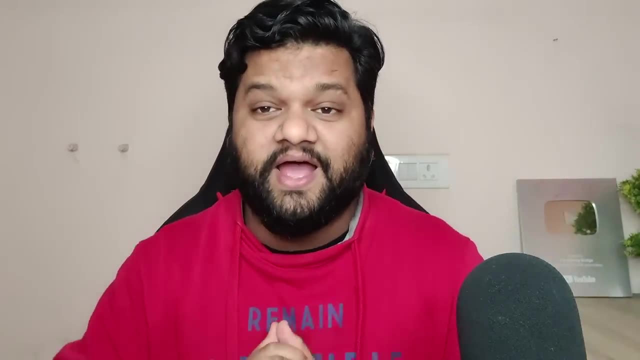 you can say data engineering roadmap 2.0. And in this roadmap video I have included my personal learnings, whole interview experiences which I've given in last two years And with the help of that one I have created this really, really extensive data engineering. 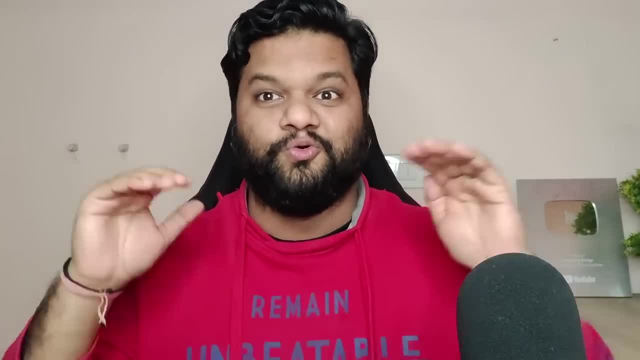 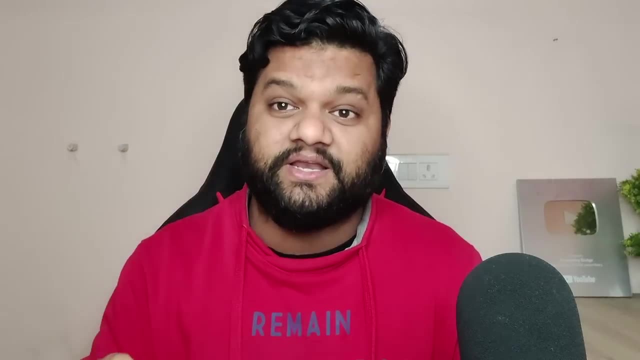 roadmap video. Once I will open it, you will be like: dude, what is this? This is so extensive, but I can honestly tell you that this is a really, really extensive data engineering roadmap video And if you follow this roadmap sincerely, thoroughly and consistently- 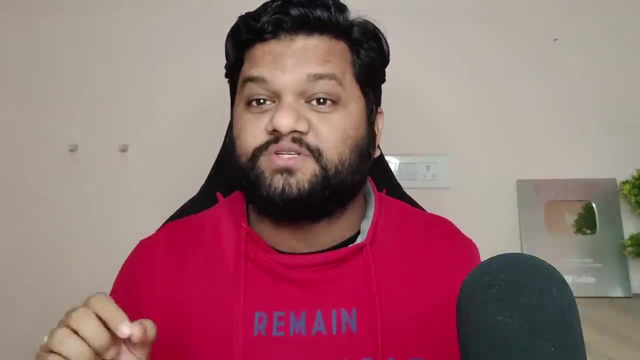 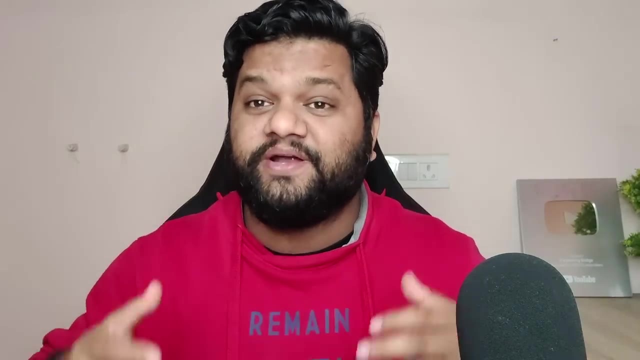 then, within a few months, you will be equipped with the most demanding skill set of data engineering. So watch this video till the very end to know the complete roadmap and share it as much as you can, so that newcomers in the data engineering can also follow this. 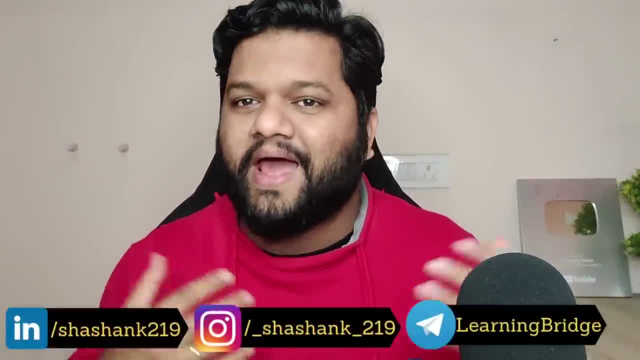 crisp and very extensive roadmap of 2023. And, as always, if you feel this is really value adding for you, then hit the like button and share it with your friends and family. Thank you so much for watching this video And I will see you in the next one. Bye. 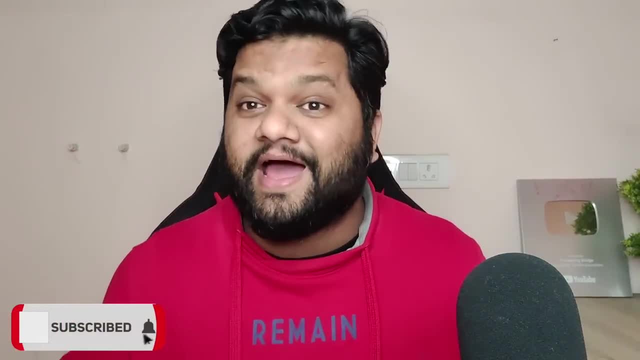 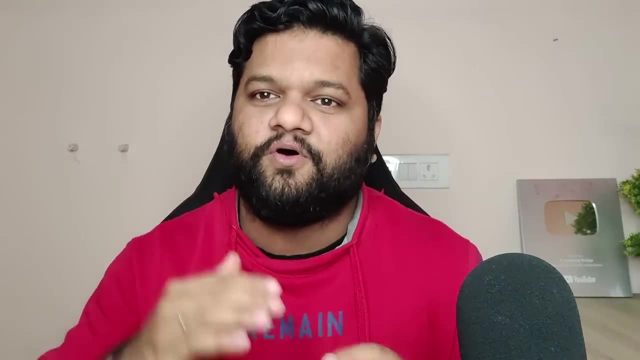 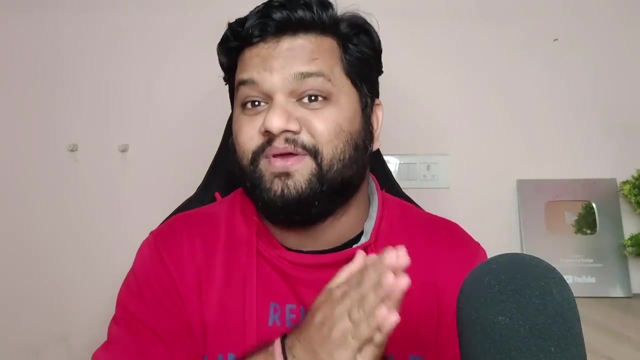 Also, after going through with this roadmap video, try to rate yourself for all these listed skill set in the comment box, so that I can know how much you have been into this data engineering journey. So I will walk you through with every single section here and: 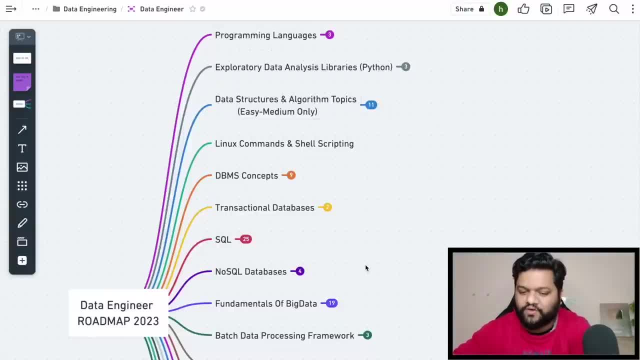 will elaborate as well This roadmap video. first of all, I have created in a sequential way, So first half of this roadmap is something Which is the fundamental, or you can say the building blocks are the base of your data engineering journey, And the first half of this roadmap video is actually very much needed. 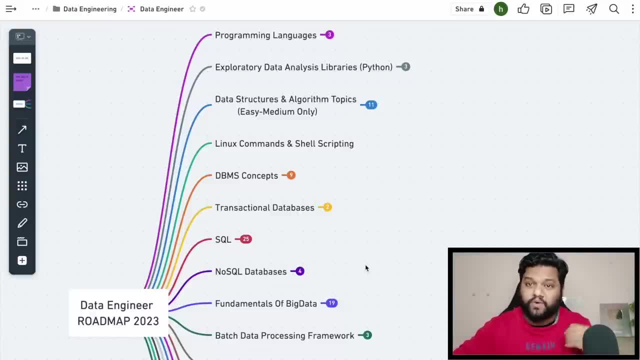 This is like across all the job description. If you are applying in tier one companies or any good product based companies, startups, service based companies, consulting firm, this is going to be the common one. So, first, starting with the programming languages and this one, you can start with Python, Scala. 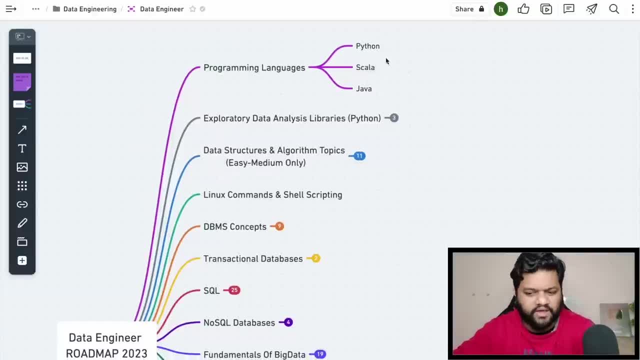 and Java And, from my recommendation side, Python, again being the language of the data. If you are starting, if you are new, then definitely start with that one, But in the data engineering space, these are the three languages which are really popular. 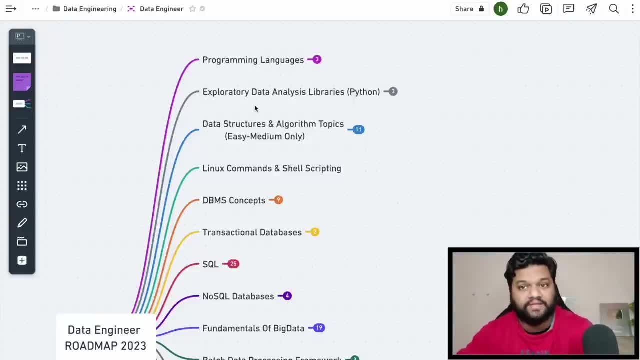 Moving on to the next section, like, if you are going ahead with the Python, then Python has a very, very rich support for all the data analysis related stuff And that is why it is very much popular. So you should also look into the exploratory. 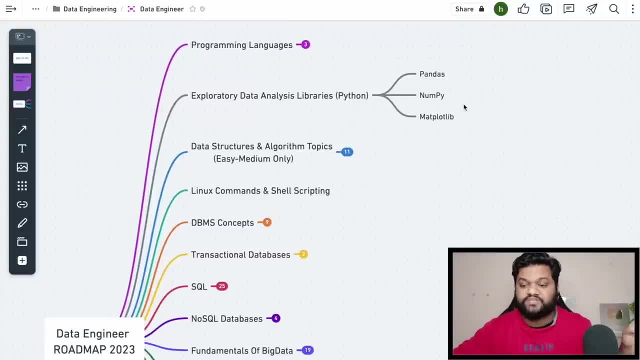 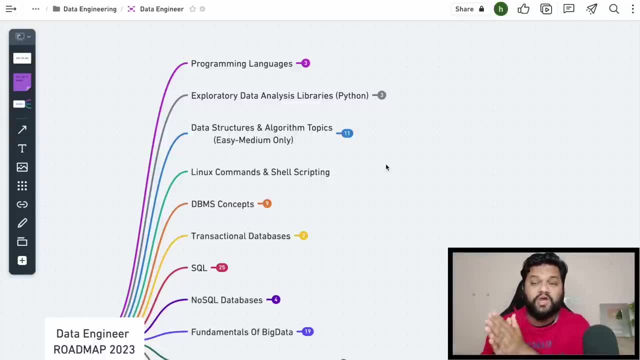 data analysis library. It is in Python, like Pandas, NumPy, Matplotlib. Now, moving on to the next part, this is the most often asked question as well: How much programming is actually needed in data engineering space for interviews, How much we need to code? 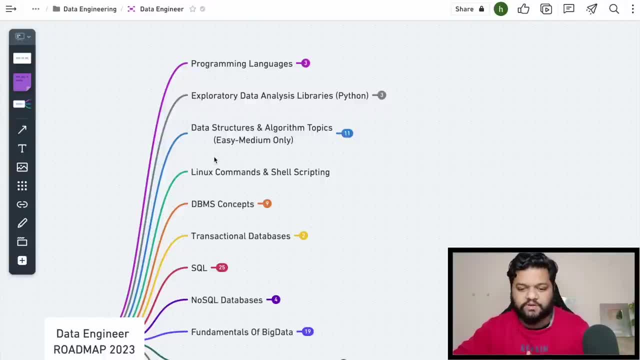 To answer this doubt. this is the simplest answer I can give. The DSA part is something which is needed: easy, easy, medium till medium, Not more than that. You do not need to be a pro competitive coder or something like that, So do not invest that much amount of time in that. 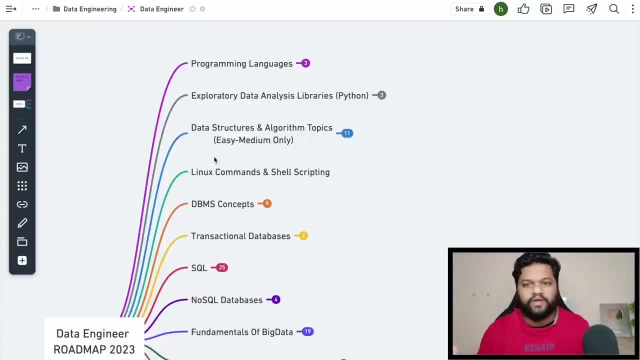 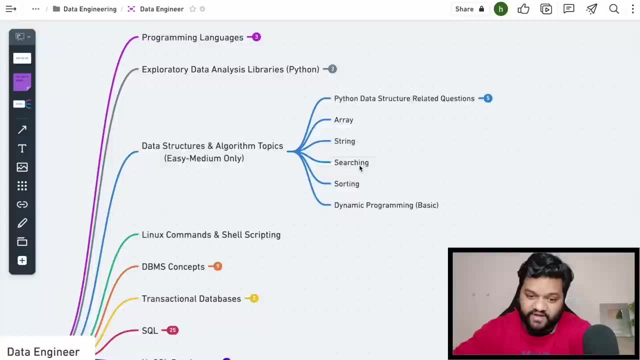 Direction. If you love solving it, keep on doing it. It's pretty good. But I'm just telling you from the interview point of view. So in this one, what all topics you should definitely cover. First of all, Python related questions you might get in the interview. 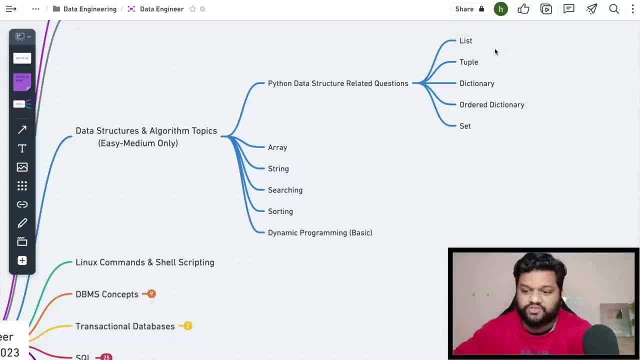 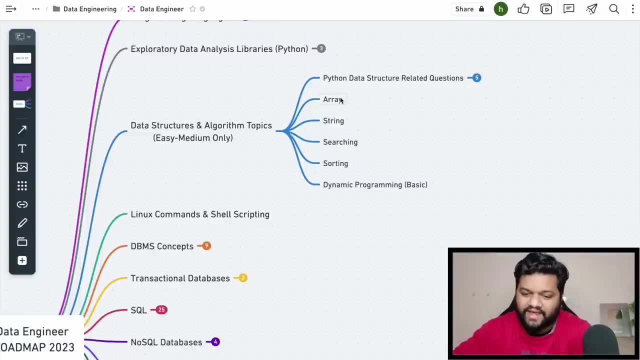 So try to cover these mandatory data structures of Python like list, tuple, dictionary, order, dictionary set. Then the generic data structures and algorithm related topics like array, string searching, sorting and dynamic programming. Then the basic or you can say easy to medium level. 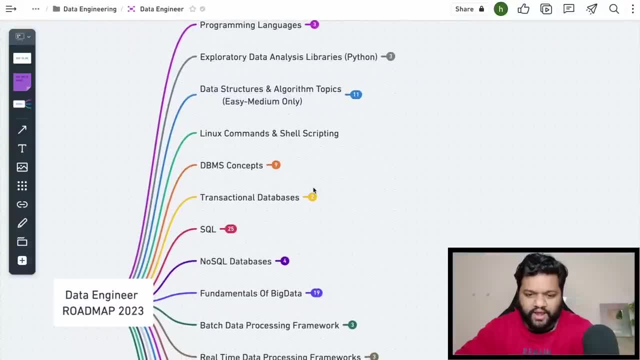 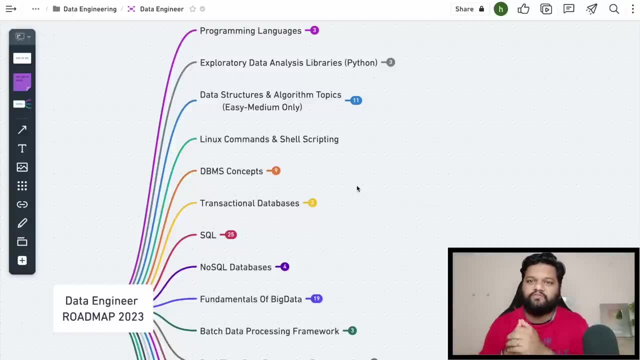 Now moving on to the next one, which is like the core, And this is the part of your day to day activities. So most of the times we will be working on these servers, like those kind of operating systems where we need to work on the command line right. 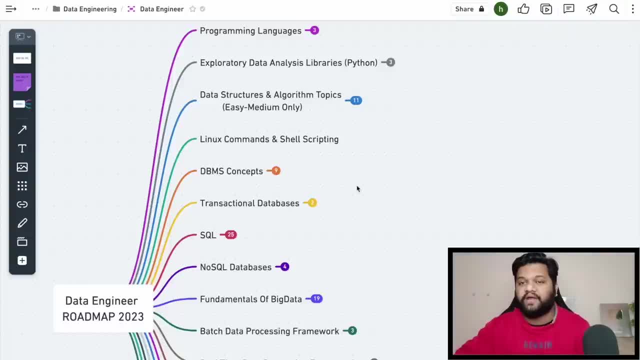 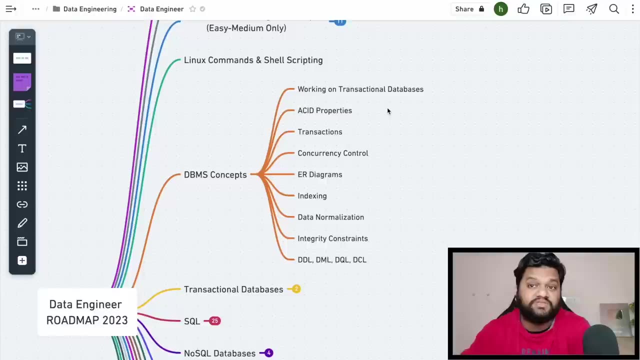 So you have to be really good at the Linux commands and writing the shell scripting, because sometimes we need to automate some jobs or any kind of stuff, So you need to know that part as well. Next part: Next part is database management concepts. So you should definitely start with the why section, like why transactional databases. 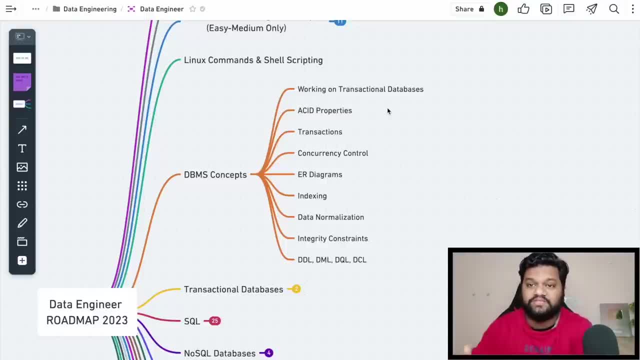 why they came into the picture. what is the actual need of them? understanding their use cases, then the core of it, like ACID properties, transactions, concurrency control, ER diagrams, indexing data, normalization, integrity constraints and the very creamy layer of SQL which will 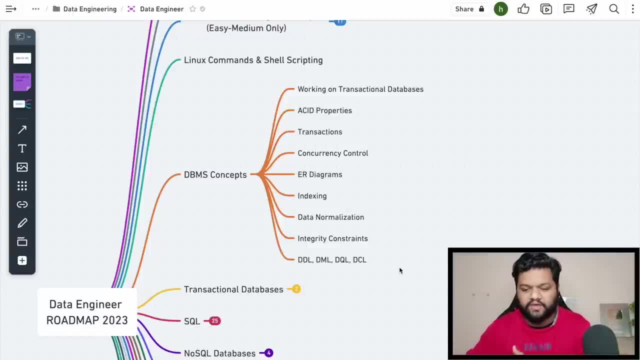 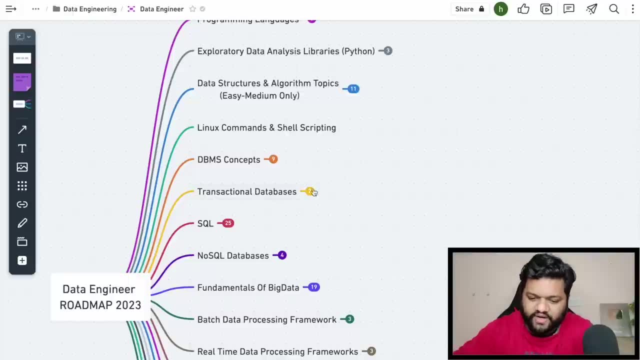 be the kickstart of it, like understanding of DDL, DML, DQL, DCL, Very basic components, Very basic commands of the SQL part, Moving on to the next one, the transactional databases. So in the industry, these are the two things which are really popular. 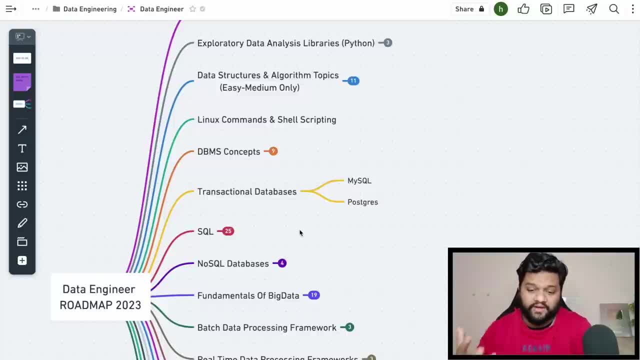 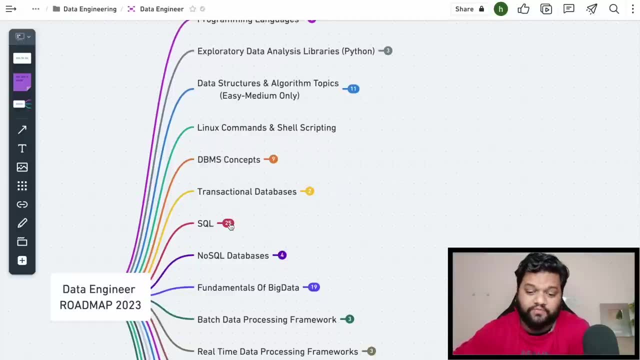 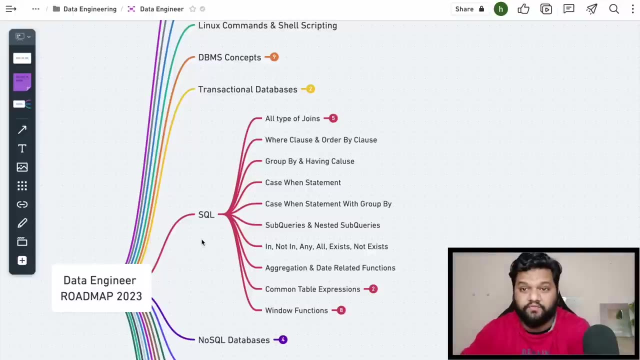 MySQL and Postgres, two very most popular transactional databases. you can say So. if you are starting with this one, try to pick any of it. Next, the bread and butter for all the data professionals, And this is the section which will have even 40% of weightage in your interviews. 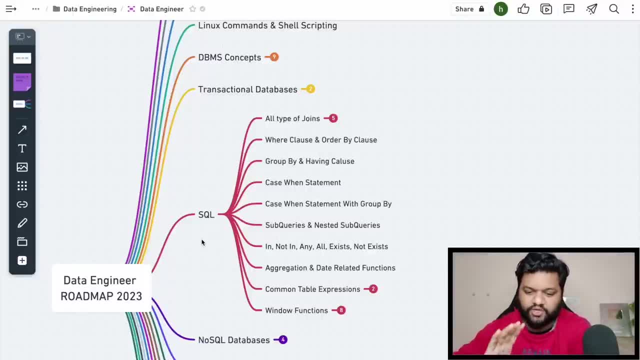 So, based on my experience, This is something you definitely need to cover, Because, as a data professional, your domain for SQL is not limited to joins and group buys only, or just a select operation- insert, delete. So in our day to day activities SQL, we use it very extensively, and not only the easy. 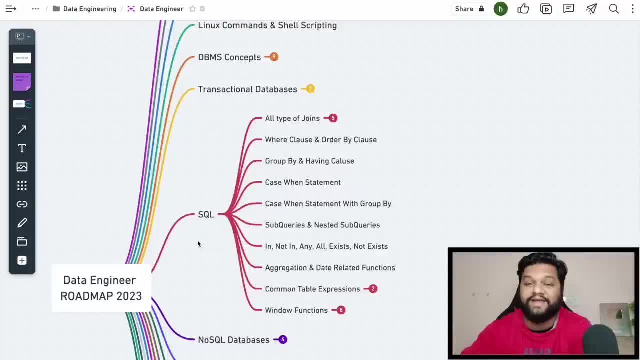 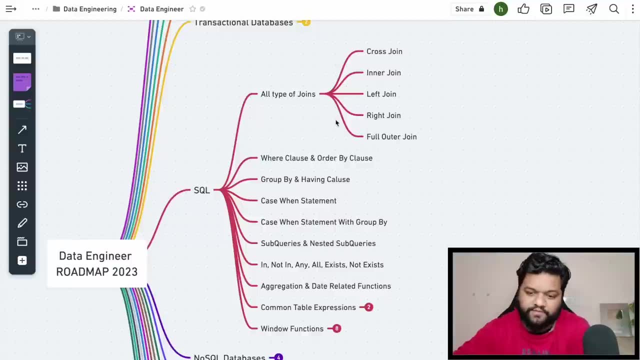 part, like including medium and advanced part of SQL for the data analysis. So these are all things you need to cover for sure. all type of joins: cross join, inner join, left right, full outer join where clause and the order by clause, group, by and. 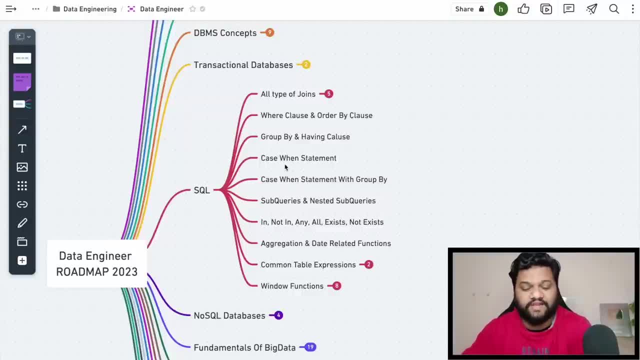 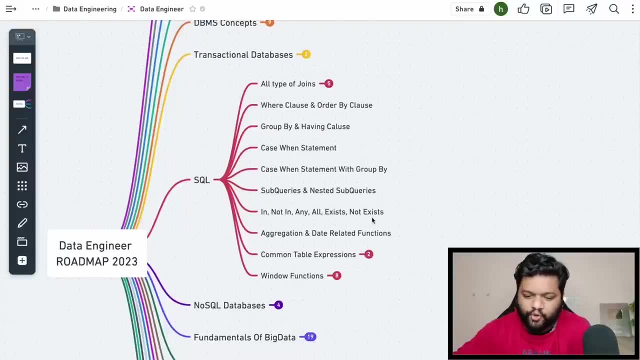 having clause case when statements, which is sort of if else kind of thing, in SQL case when statement with group buys sub queries, nested sub queries And these are some lookup related operations in not in any. all exist, not exist aggregations. 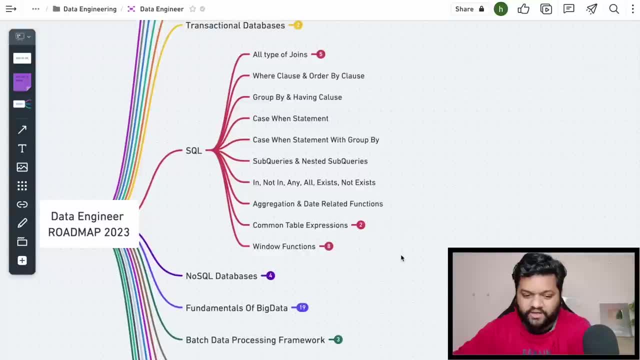 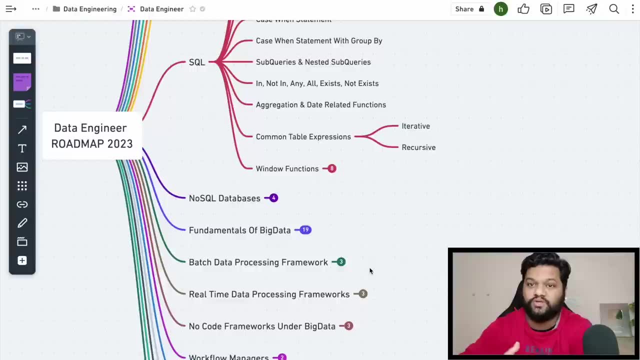 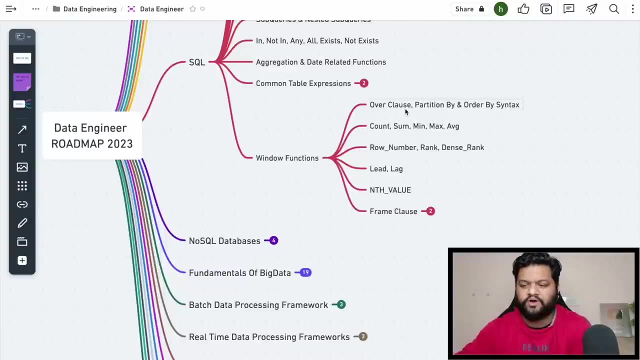 and data related functions. very common, right, we use it very frequently. then common table expressions, Like iterative common table expressions and recursive, which is eventually the with clause And then super most important window functions. So here, like over clause, partition by order, by related syntax, all the aggregation functions. 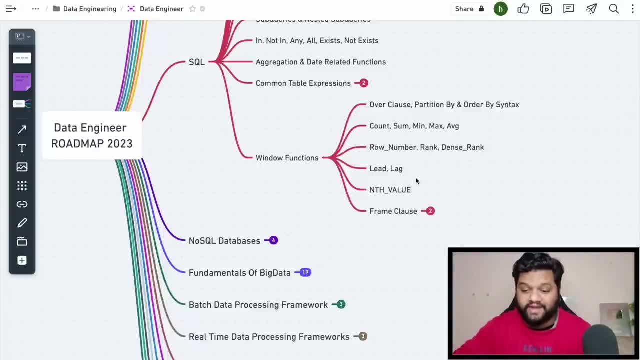 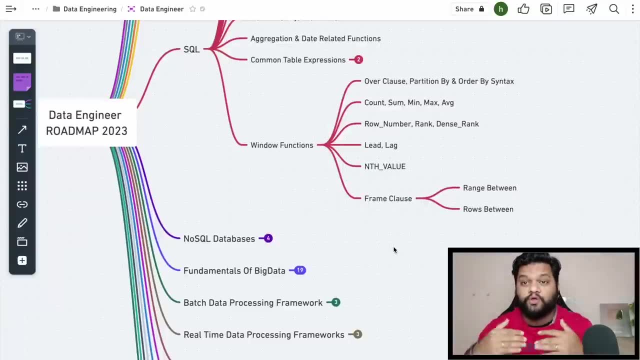 ranking related functions, very, very much important: lead, lag, nth value and then frame clause, like range between rows, between, which will help you to solve the queries which are related to cumulative sum, running sum, Running average or weekly running sum, these kind of cases. 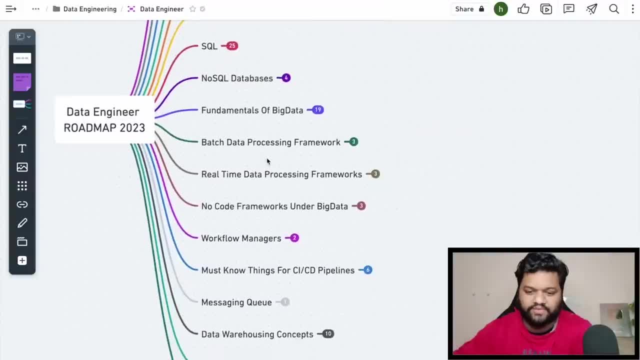 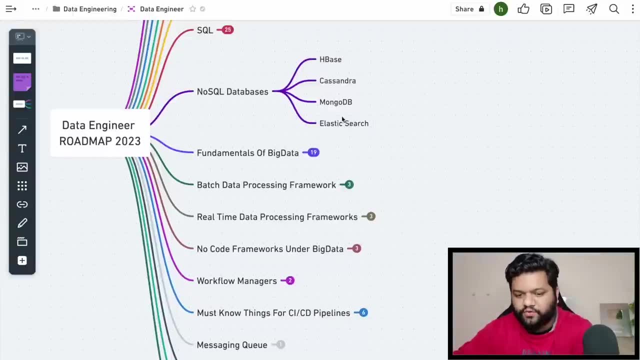 Now moving on to the next one, which is no SQL databases- again super important part of the big data space. So you can definitely look for these kind of no SQL databases. first try to understand it, understand the basis based on the CAP theorem and then pick any of the no SQL database to. 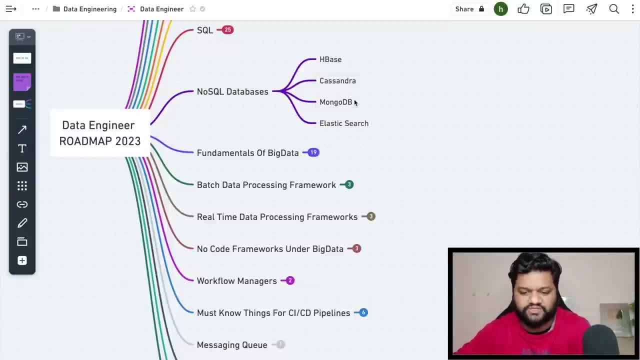 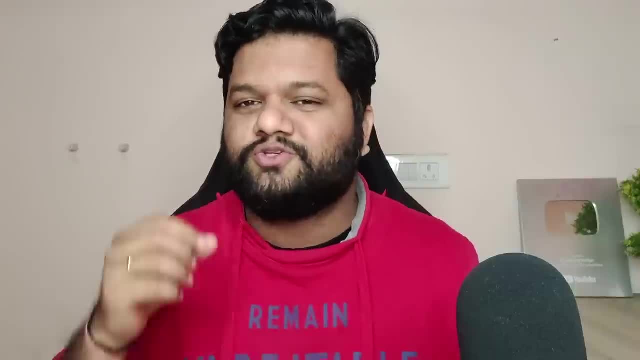 start with, like HBase, Cassandra, MongoDB, Elasticsearch. Now, till this point, We have covered the first half of the mandatory skill set for the data engineers. So if you are a software engineering enthusiast and in 2023, you want to invest in your future, 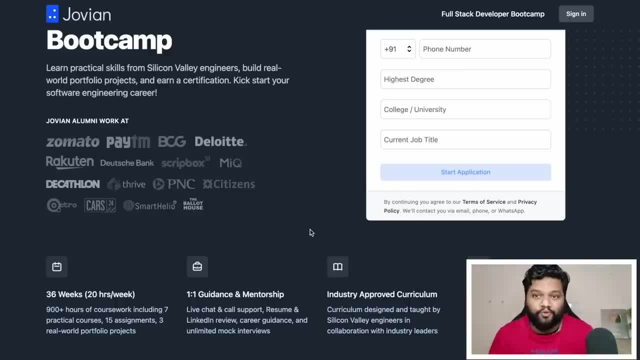 and I would highly recommend to join Zovian full stack development bootcamp. their alumni are working in top multinational IT firms and have backed the package ranging from six lakhs to 40 lakhs per annum. This would be a 36 week long bootcamp where you will get 900 plus hour of content, including 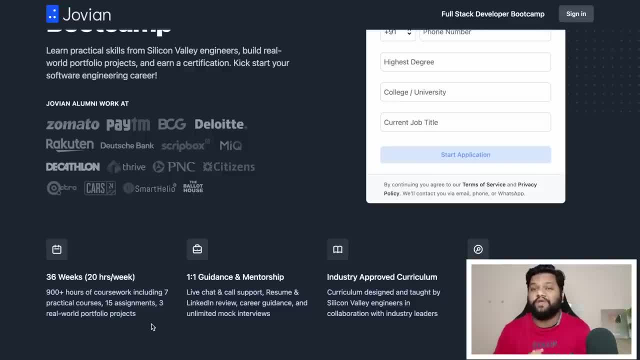 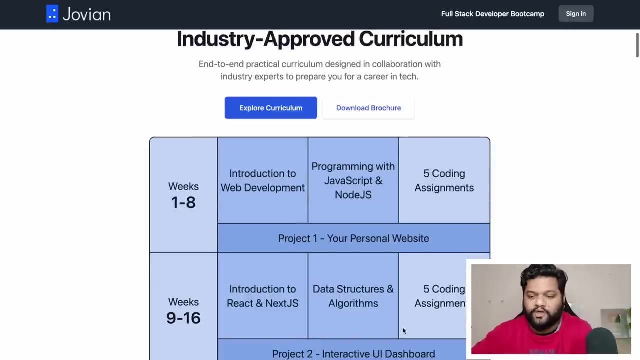 seven practical courses, 15 assignments and three real world projects. One on one mentorship will be provided for resume, LinkedIn, career guidance and unlimited mock interviews. They have an industry approved curriculum which is designed by the top notch Silicon Valley engineers. you can look at the curriculum, where you will be taught the latest tool and 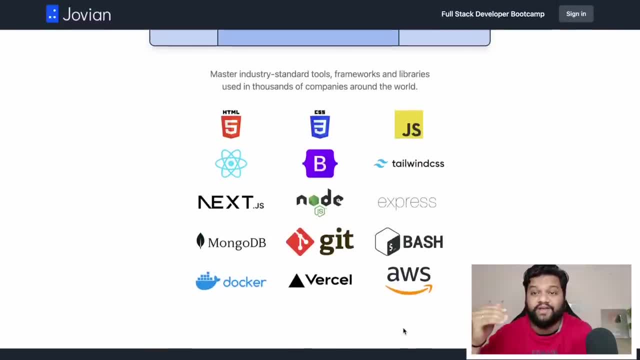 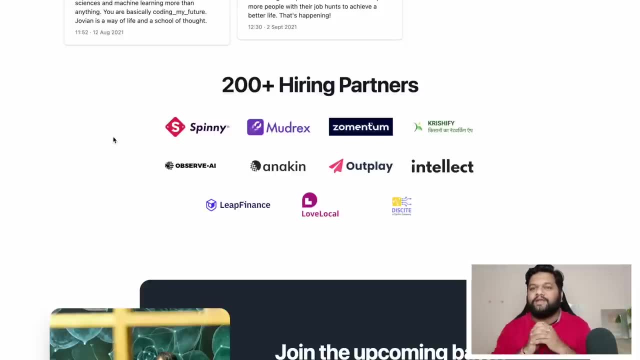 tech frameworks which are highly, highly demanded in the industry right now. The mentors of Zovian are actually leading industry experts and this is the full job guaranteed program Where you can get Hired by 200 plus hiring partners on boarded on Zovian within the 12 months of your graduation. 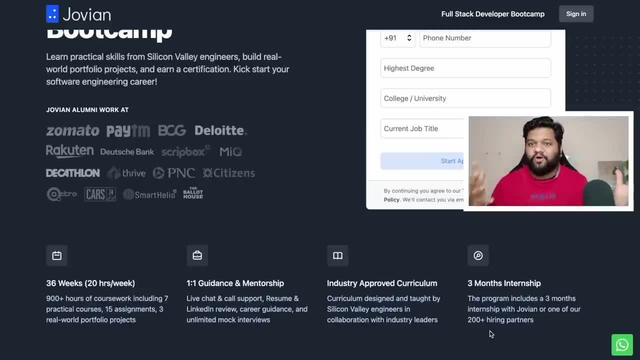 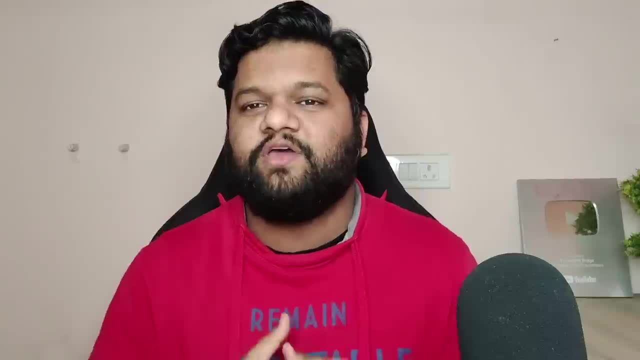 And this program also includes three months of internship at Zovian or any of their hiring partner. So far, thousands of learners have transformed their career with the help of Zovian. I have given a link in the video description. Their new bootcamp is starting really soon. 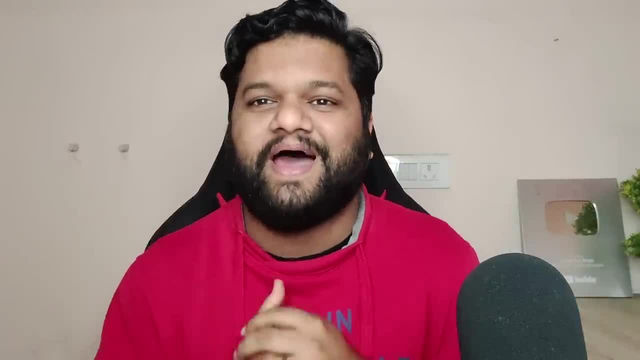 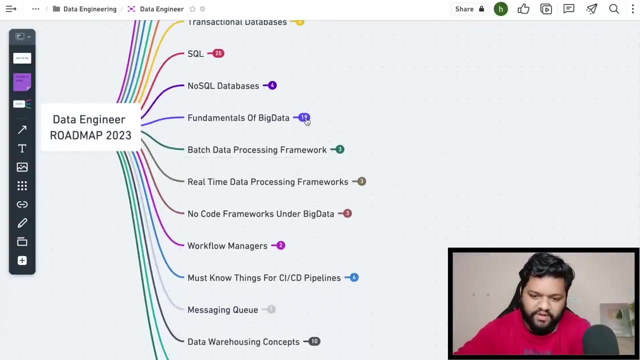 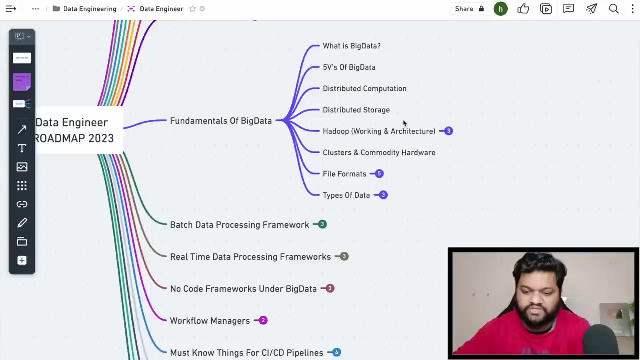 Also, they have a no cost EMI option as well. hurry up and enroll in this program Now going into the depth of big data. So first you should start with the fundamentals, the things you need to cover. What is big data? five V's of big data: distributed computation, distributed storage, Hadoop, like. 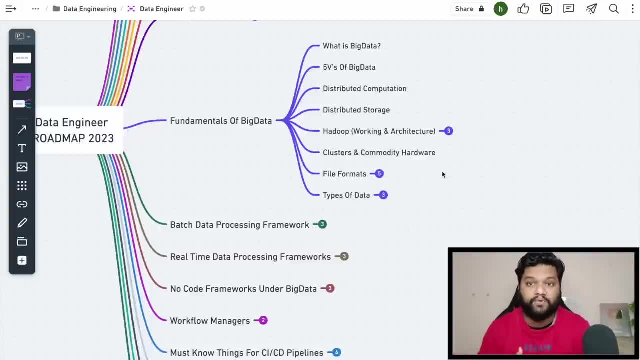 this is the first framework which came into picture for the distributed computation and distributed storage. So you do not need to deep dive into the programming part of Hadoop, right, Because we have a lot more improved and advanced distributed computation engine, but their base is definitely Hadoop. 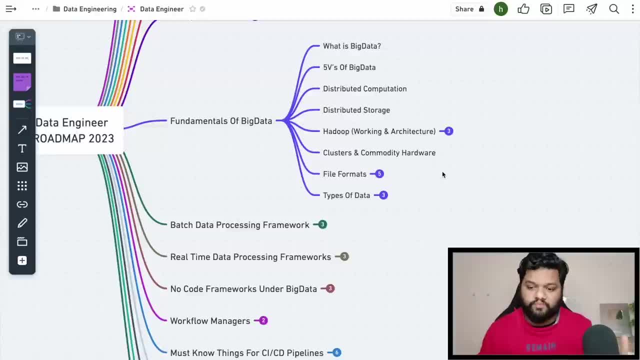 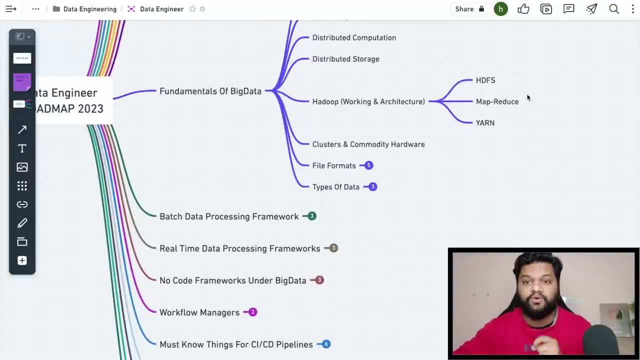 The methodologies. They are based on Hadoop. This is definitely adapted from the Hadoop, So you need to know it's working and architecture in depth, Every single segment of it, like HDFS, MapReduce, and resource management, like Yarn. 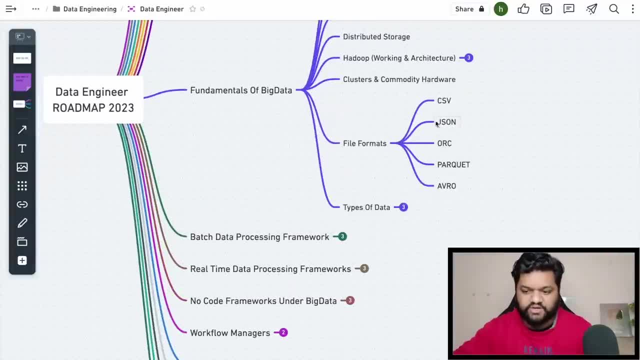 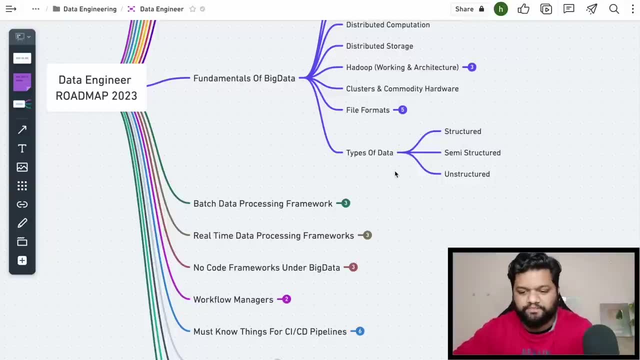 And then clusters and commodity hardwares, file formats. These are like CSV, JSON, ORC, Parquet, Avro, types of data like structured, semi-structured, unstructured. Moving on to the next one, which is batch data processing framework. 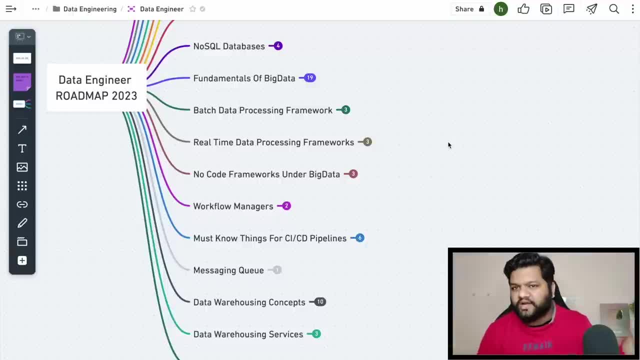 So in big data mostly we have three segments. So this is like batch data processing, near real time data processing and real time data processing. So for batch data processing, the framework you should definitely target and this is the mandatory skill set nowadays, right? 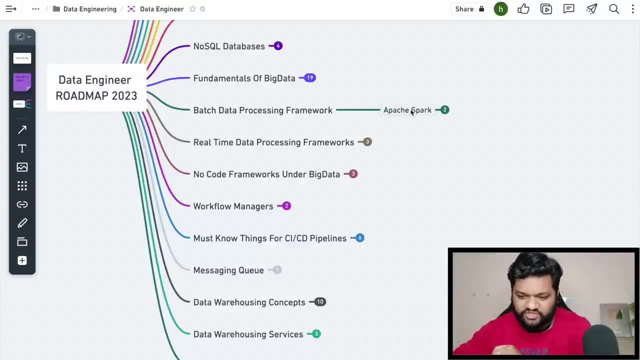 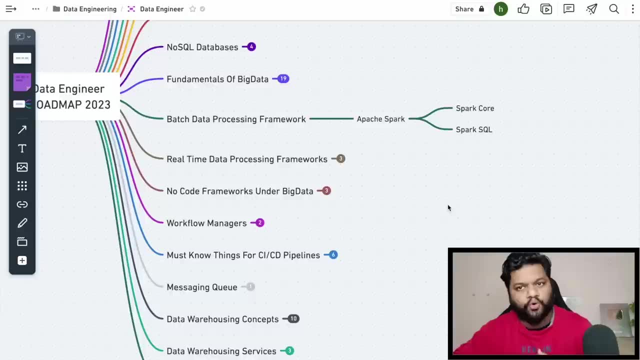 This is the mandatory skill set for the data engineers Apache Spark. So, with respect to batch data processing, these are the two segments you need to cover from the Apache Spark, like Spark core and Spark SQL. Now moving on to the next part, which is related to real time data processing. 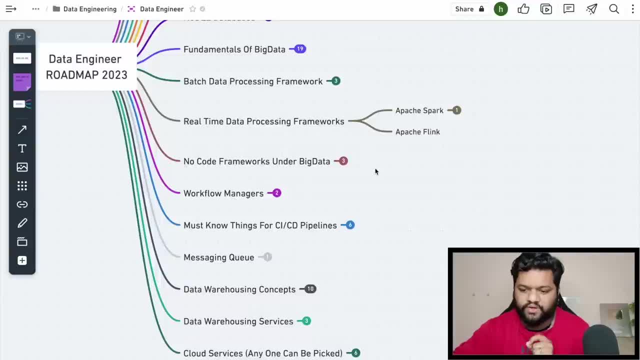 So this is the mandatory skill set for the data engineers: data processing frameworks. so for this one- apache spark- the spark structured streaming- you need to focus. and next one, which is apache fling, which is getting really, really popular when it comes to create pure real-time data streaming pipelines, and since i have been using it personally for 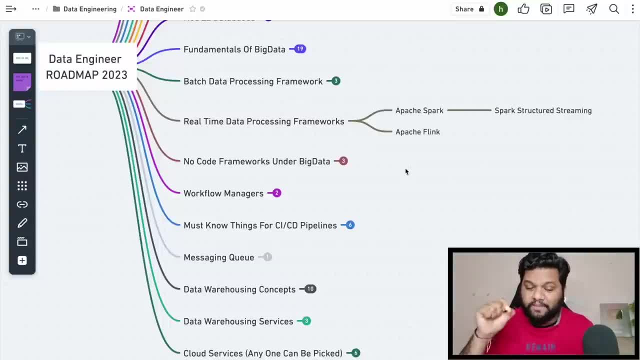 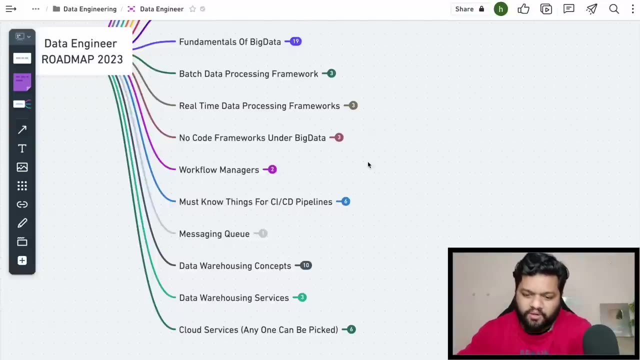 production level applications. i know how much amazing this is, so make sure for this sort of use case. you must try this and you must explore it, and lots of companies are asking it in their job descriptions. moving on to next one: no code framework under big data there are popular no. 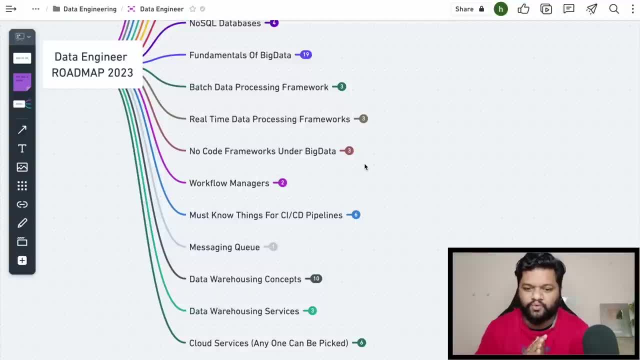 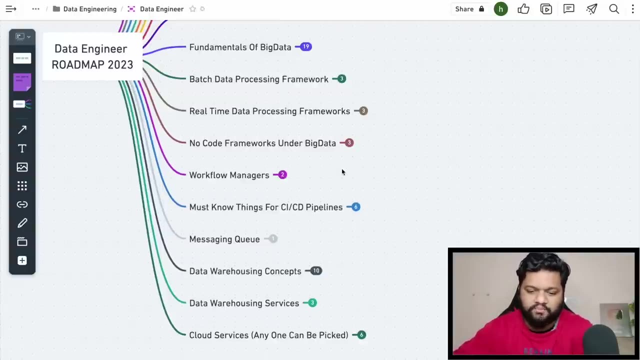 code frameworks means where mostly you need to work on the configuration basis and the drag and drop kind of features to build your atl pipelines. so for this one you can explore apache 9.5, apache flume and apache scoop. now coming back to the another important part, which is scheduling our 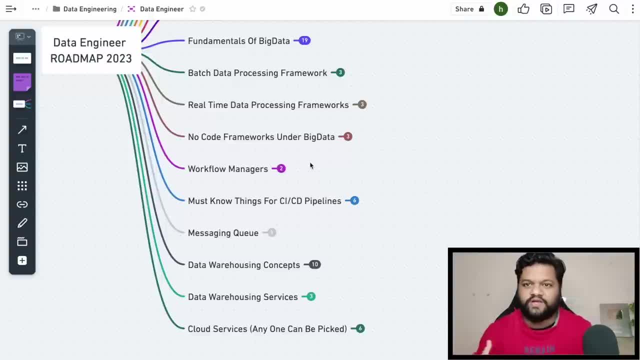 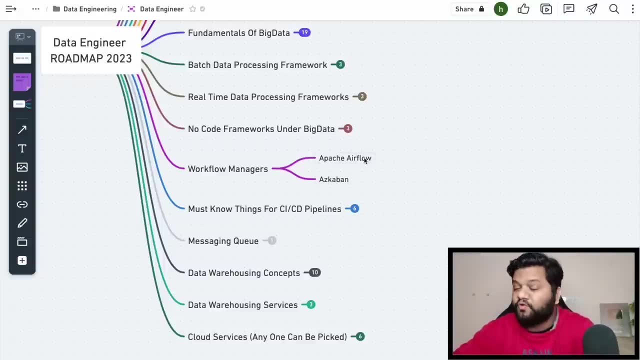 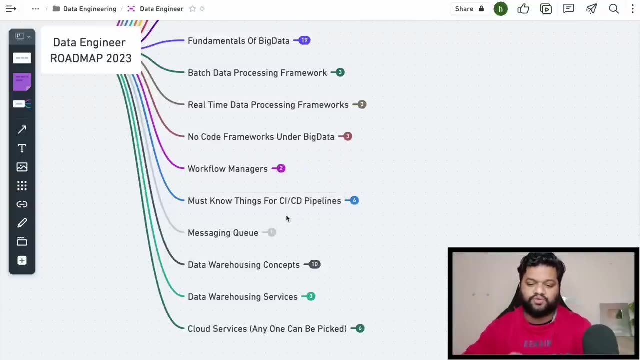 workflows, scheduling our jobs or the orchestration dependency management. so for that one workflow managers like apache airflow, azga ban, apache airflow is something which is really demanding, so you make sure you have a good, good understanding of it now must know things for the cicd pipeline: continuous integration and continuous 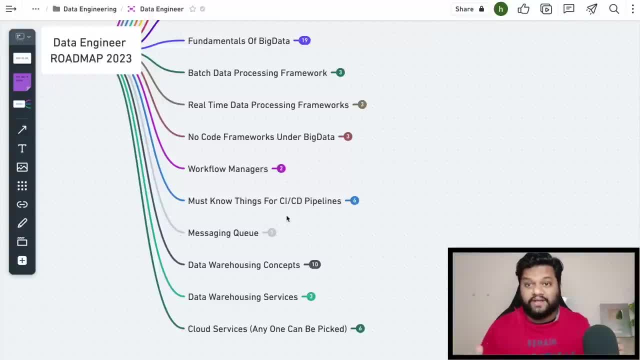 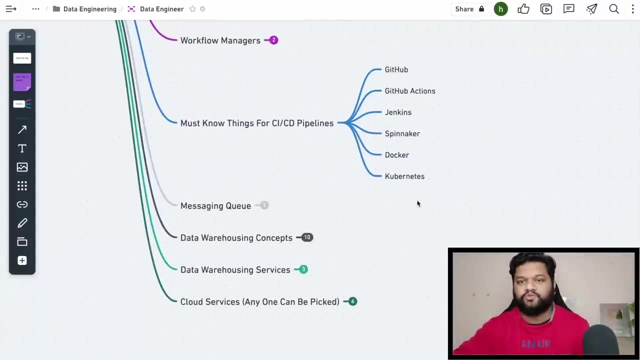 deployment. so, based on my personal experience, so far at least in this last two years i have used this sections very, very extensively right, and i will definitely show you what is inside that one. but mark my words, if you have these things in your resume and in your 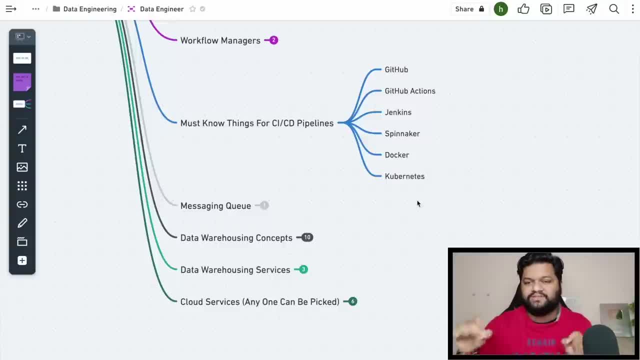 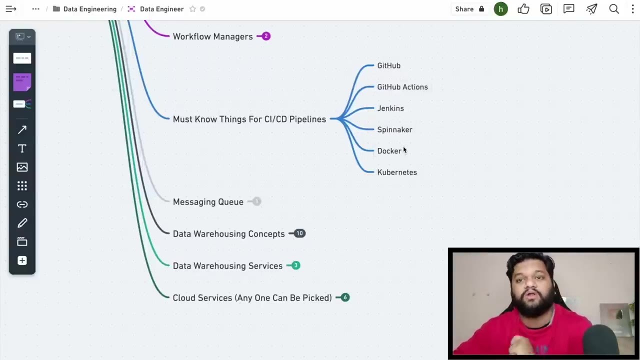 skill set. i mean you are definitely truly inside the data engineering space because when it comes to the modern software engineering or modern data pipeline development practices, these things you will definitely encounter. so github, github action, jenkins, spinnaker, docker, kubernetes- so that's why i have mentioned, must know things for cicd. 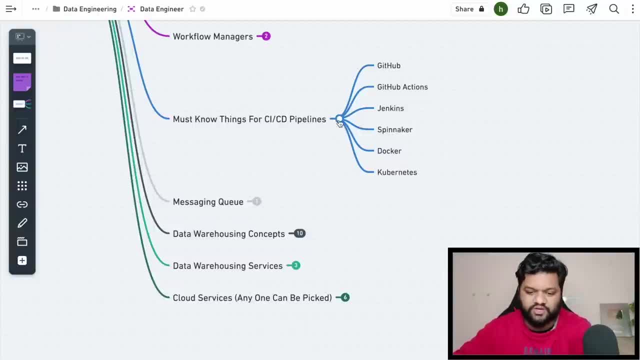 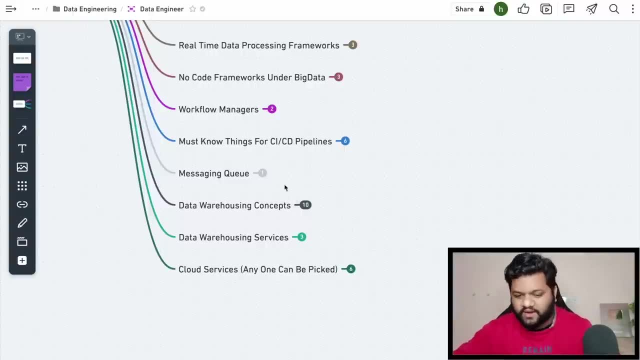 pipeline, and this would be the expectation from the data engineer. now the messaging queue part which would be needed to build the streaming pipelines. and again, my personal experiences: apache, kafka: i have been using it very, very extensively, so you should also have a really good understanding of it, deep dive it and build applications around it. now, data warehousing. 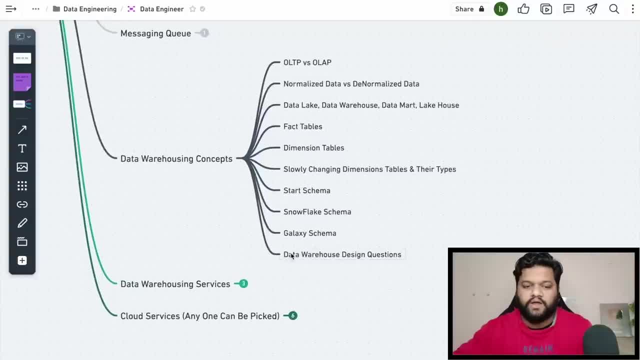 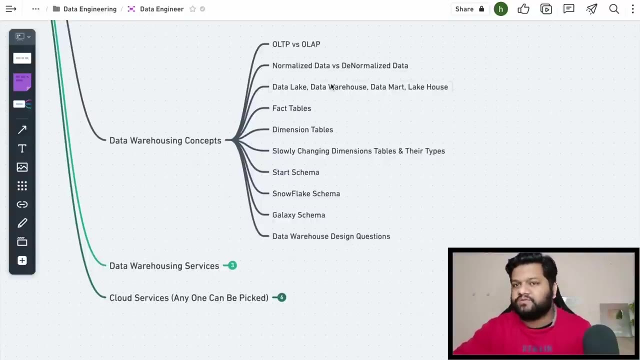 concept again a very, very important part for the day-to-day activities, plus interview experience and, most specifically, if you have three plus years of experience, then in your interviews this round would be super important. so in this one, olTP versus OLAP, normalized data versus denormalized data, lake. 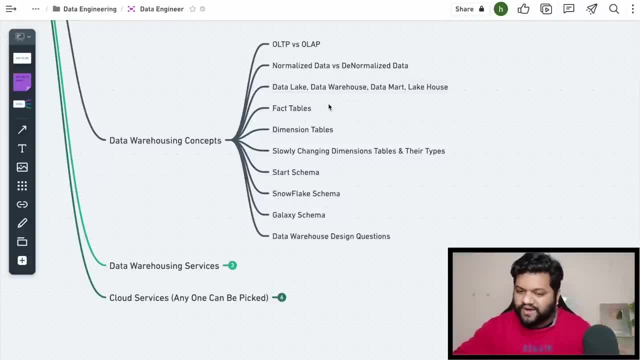 data warehouses: data mart, lake house. what is fact? table dimension table slowly changing dimension table, their types, star schema, snowflake schema, galaxy schema and real world use cases around the data warehousing. this is how you will be getting your data warehousing and data warehousing experience. 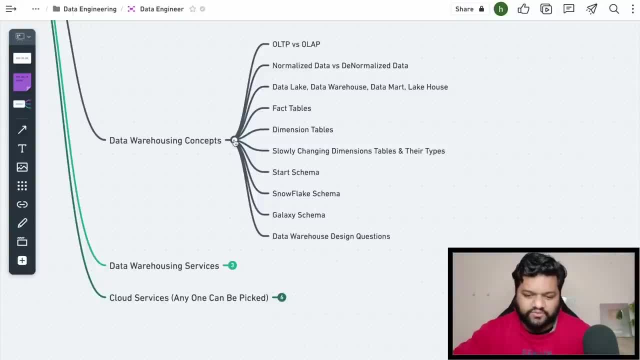 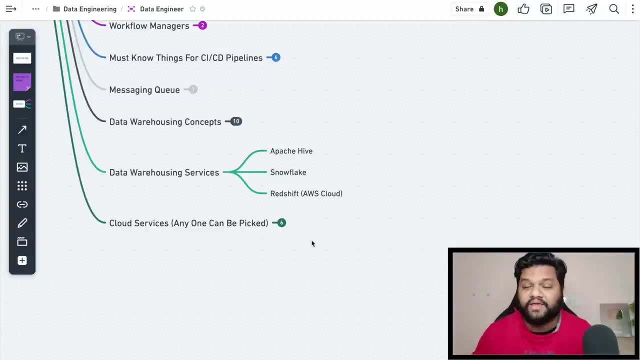 getting your questions in the interviews. So data warehousing concept. Next one, data warehousing services like those frameworks which are really, really demanding in the industry when it comes to the best data warehousing solution. So Apache Hive is there as an open source Snowflake getting a lot, of, lot of popularity. 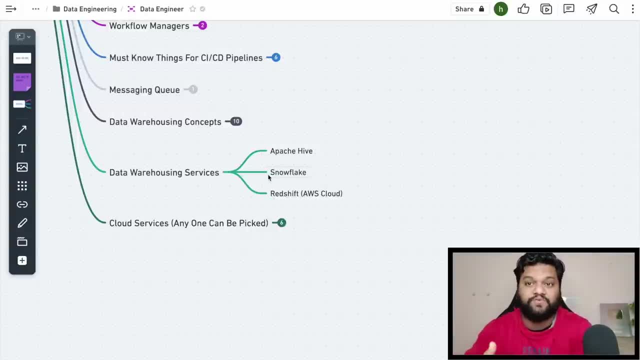 and you will even find the job profile specific to this one Snowflake developer. So this is something which you should definitely target in 2023 and, when it comes to these data warehousing services with respect to the cloud, AWS, Redshift is definitely dominating at this moment. 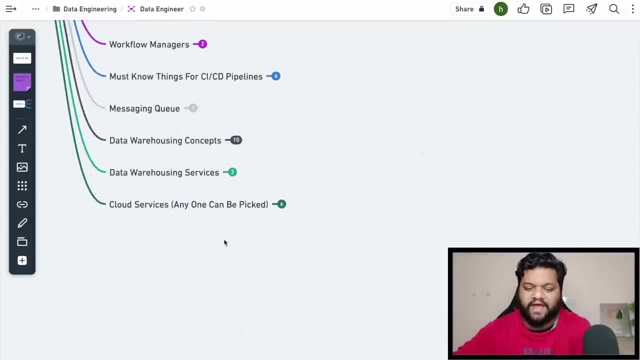 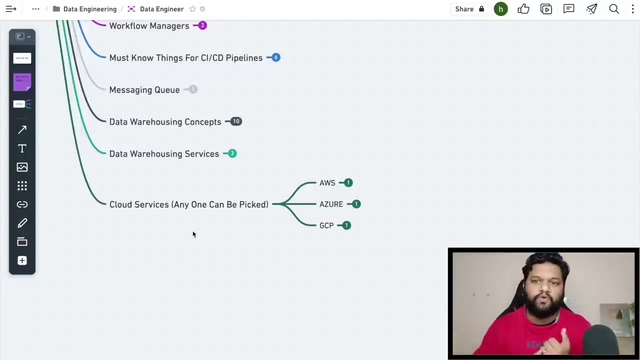 So now coming back to the last but not the least and match made in heaven, which is cloud services plus big data. So I have created the three segments because at any given point of time, you can start with any of the cloud components. But if you look at the market, if you look at the job description in most of the companies, you will find AWS is there as their primary cloud platform. As a beginner, you can definitely start with any one which you feel feasible, So I have listed down the important services which you need to target with respect to data engineering, big data and data pipeline building for every cloud platform. 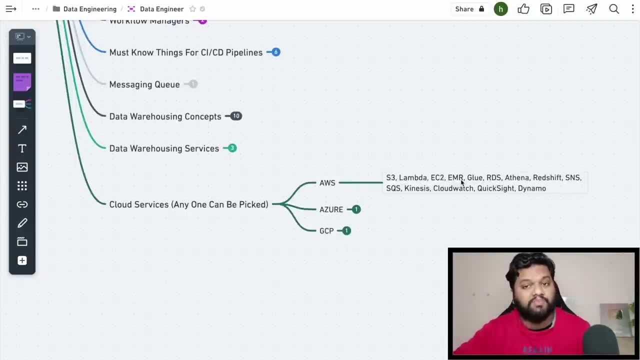 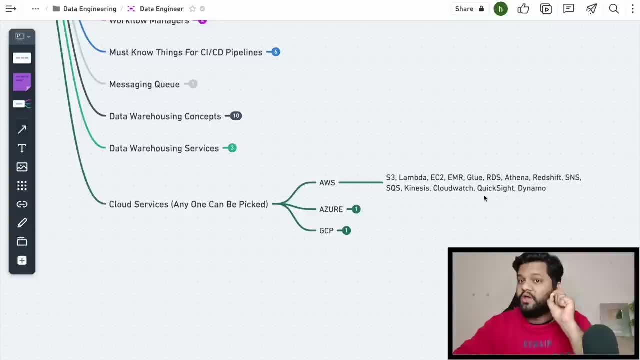 Azure, Azure, Azure, Azure, Azure, Azure, Redshift, Redshift, SMS, SQS, Kinesis, Cloudwatch, Quickside and DynamoDB. These all things you should know if you are starting with AWS. coming to the Azure part, 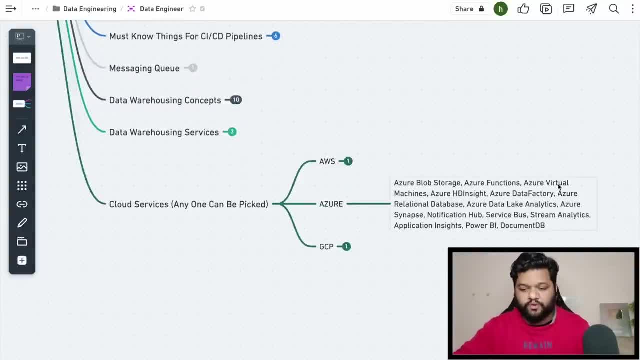 here: Azure blob storage, Azure Functions, Virtual machines, HD insight, Azure Data factory, which has gained a lot of popularity. I must say so: if you're starting with Azure, make sure you have a very, very strong knowledge of Azure Data Factory as your relational databases. 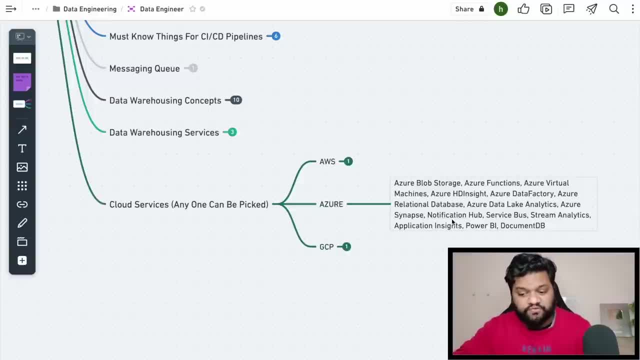 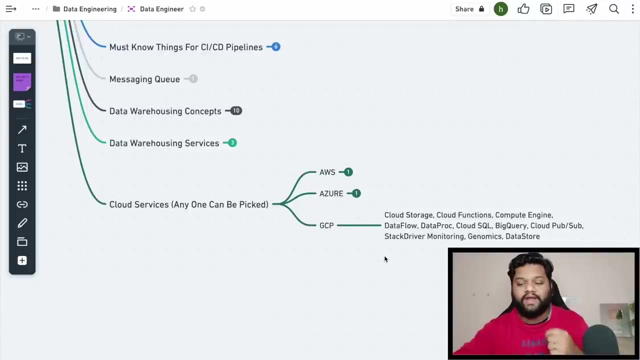 databases, data lake analytics, azure synapse, notification hub service, bus stream analytics, application insight power, bi document db. so that was about the azure. coming back to the gcp, so cloud storage, cloud functions, compute engine, data flow, data proc cloud, sql, bigquery- popular service from the gcp side when it comes to the big data cloud, pub sub stack. 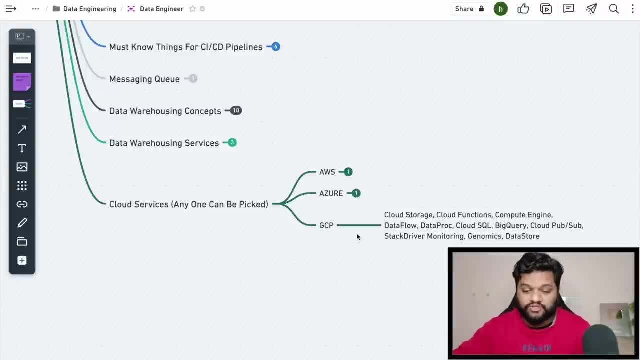 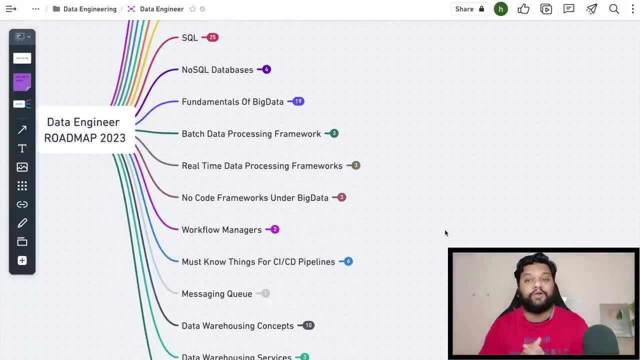 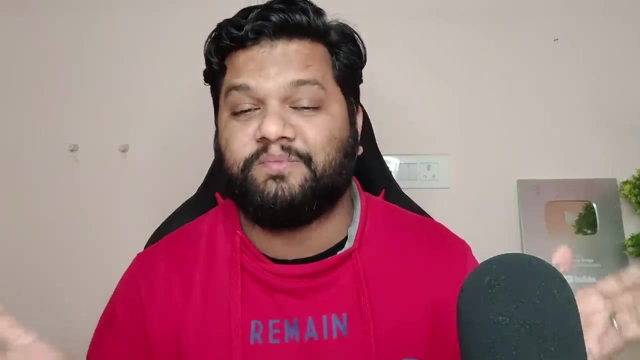 driver monitoring, geonomics and data store. so that was about the cloud services and that was even the end of our data engineering roadmap 2023.. as i mentioned in the beginning, when you will open this roadmap video, this will look super extensive, but that is the beauty of this roadmap, so i hope. 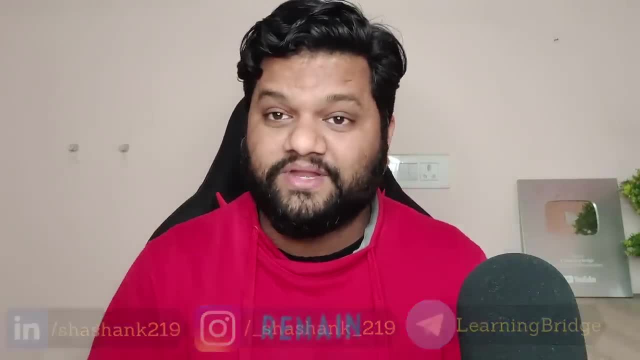 this would be super, super helpful for everyone who is starting with data engineering or who is in the data engineering but still lacking in the most demanding skill set. so you should definitely follow the link in the description box below if you are interested in learning more about data. 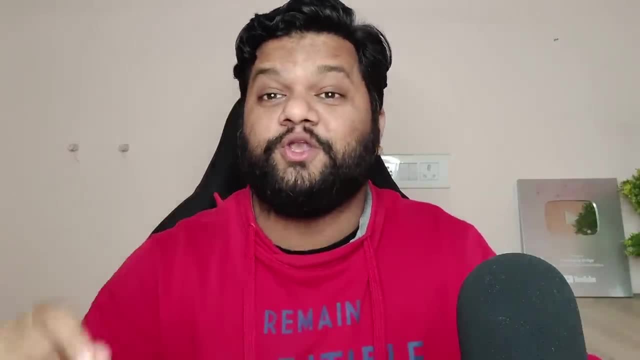 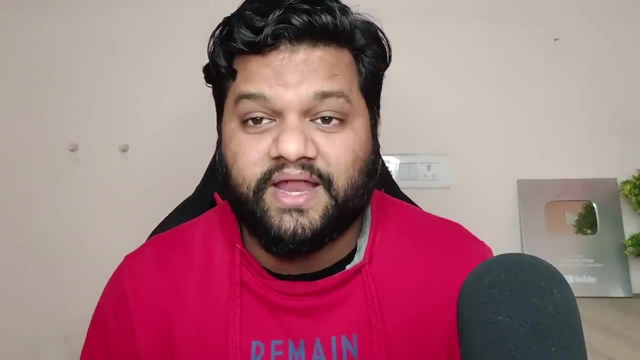 engineering, and if you feel that this roadmap video is going to help you a lot, then please drop a like, and don't forget to put your ratings for each of the skill set in the comment section. so i hope you guys would have enjoyed this video and i will see you guys in the next week with 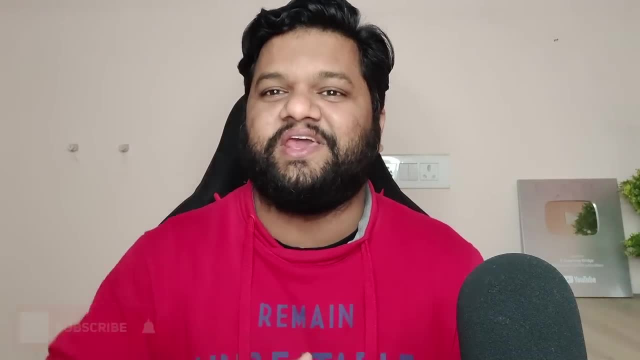 something amazing in the data engineering space. till then, just keep exploring data. so before starting the next segment of our data engineering roadmap, i want to talk about something really important.